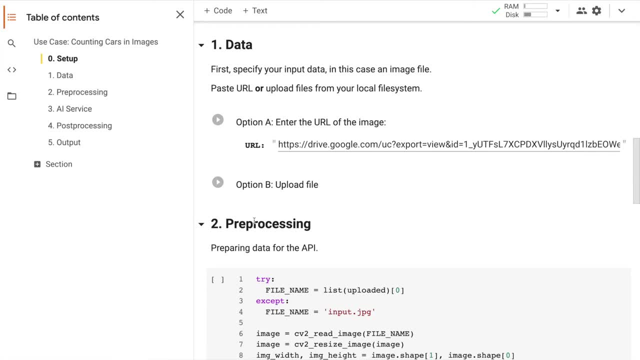 image. You can either specify an URL or upload a file from your disk. In this case, I'm using the demo image provided by this device. In this case, I'm using the demo image provided by this default URL. Run the cell to fetch this image accordingly. You should now see the file on the 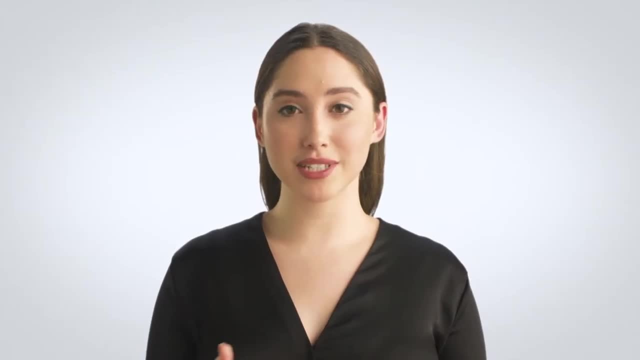 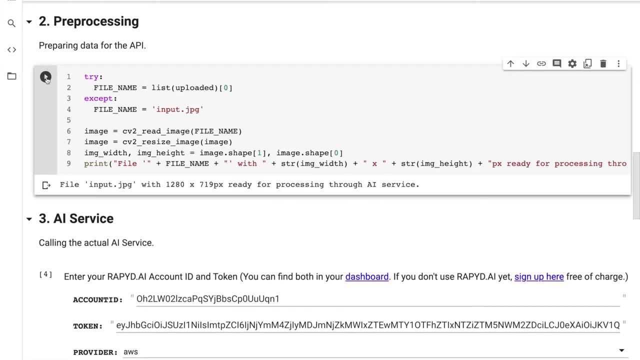 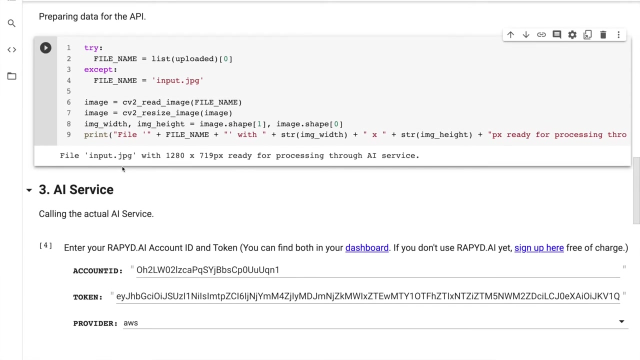 left side of the screen. Next, let's move on to the preprocessing steps For this. execute the next code cell. In this case, we want to handle the image size and make sure it's not exceeding the maximum allowed file size or image dimensions. Once this is finished and we see this little, 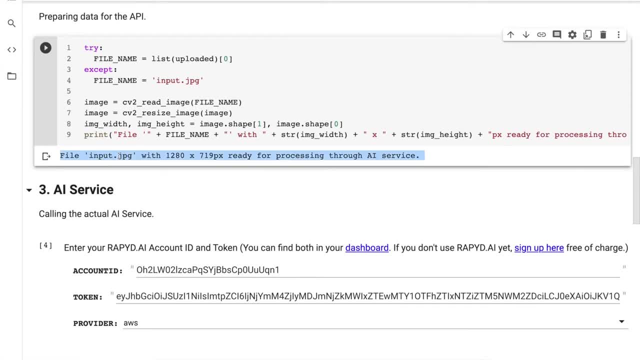 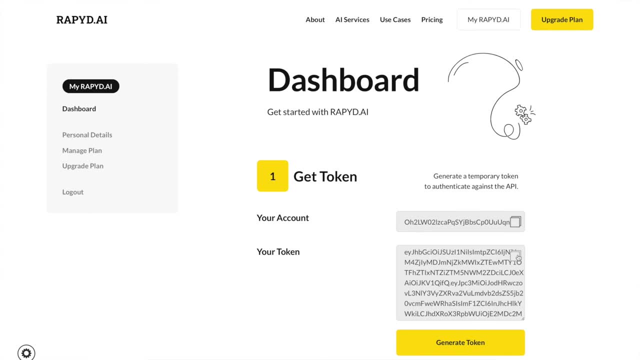 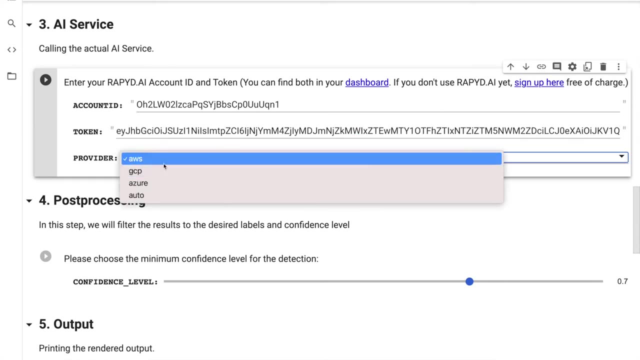 message here we are ready to call the actual AI service. Go to step 3 and provide your account ID and access token. You can find both in your rapid AI dashboard. Finally, choose your desired AI service provider. I'm going with AWS Here. it stands for the Amazon Recognition Computer Vision. 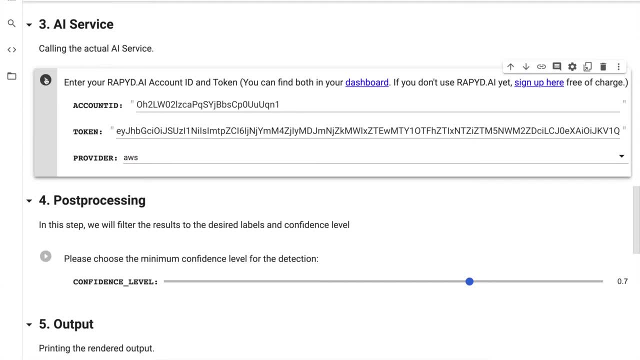 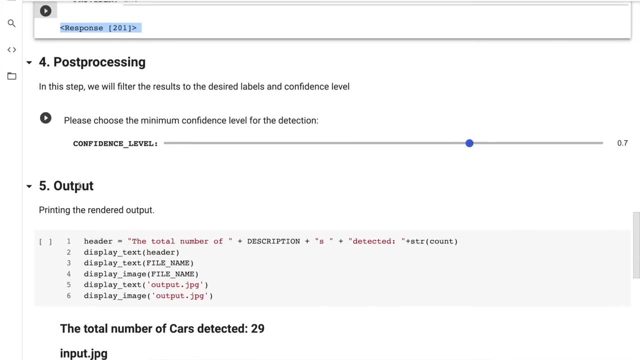 Service. Execute the cell and wait for the result. It should return a successful 201 message. Next let's head over to the post-processing stage, where we want to apply a filter and a minimum confidence score for our prediction To change the filter label. 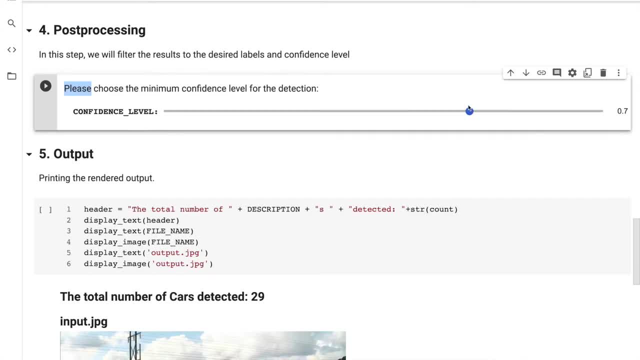 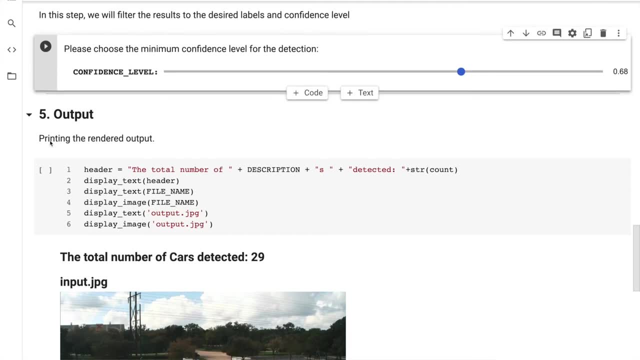 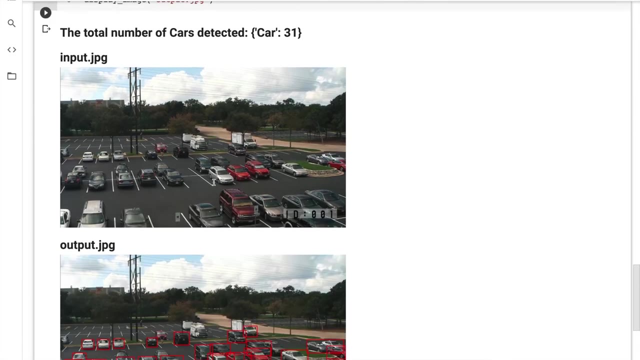 double-click the cell and modify the label variable here as you like. To adjust the confidence threshold, you can use this simple slider, Hit execute to apply the preprocessing. Finally, in step 5, we want to see the actual result. Run the remaining code cell and you should see the total image count and where your label was found. 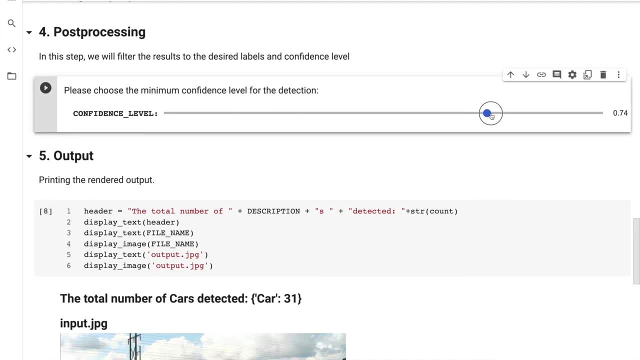 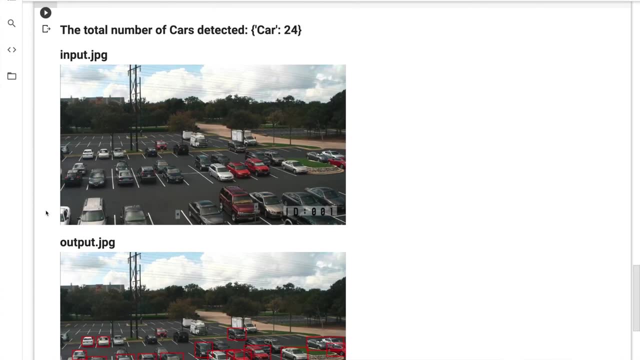 in the image. If you want to adjust, let's say, the confidence score, you can simply go back to the post-processing, adjust the confidence score, run the code cell and display the output like this: This operation is not going to call the API again, as it is just processing the AI response. 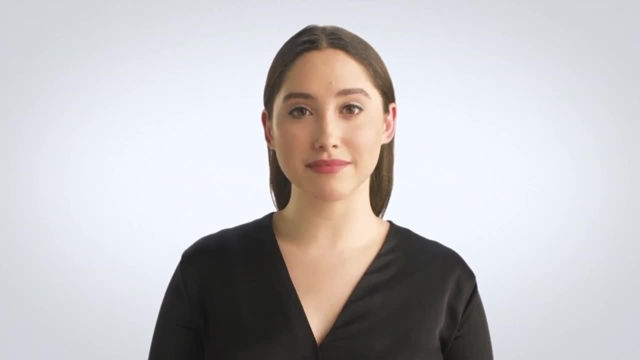 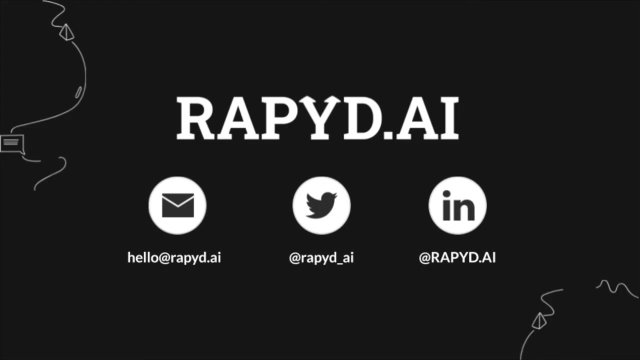 object offline. Go ahead and try it out for yourself. We hope you enjoyed this tutorial. If you have any questions, feel free to reach out anytime and we'll help you getting started. Enjoy your next AI project and see you soon.